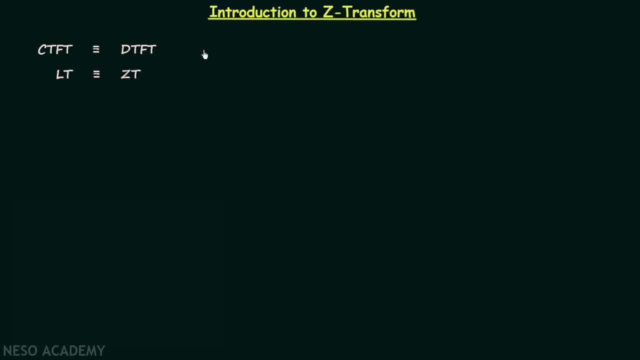 From this lecture we are going to start a new chapter and the chapter is Z transform and we have already completed continuous time Fourier transform and the Laplace transform. and we know we use CTFT to convert continuous time domain signals to their corresponding frequency domain representations and we use CTFT to analyze the continuous time signals. 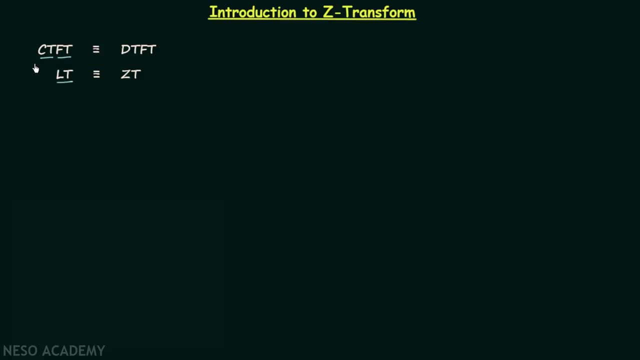 On the other hand, Laplace transform is the general case of CTFT and we use Laplace transform to analyze continuous time systems. We can comment about the stability, causality etc. of a continuous time system using the Laplace transform. Now we will talk about the existence of CTFT. CTFT will exist for energy. 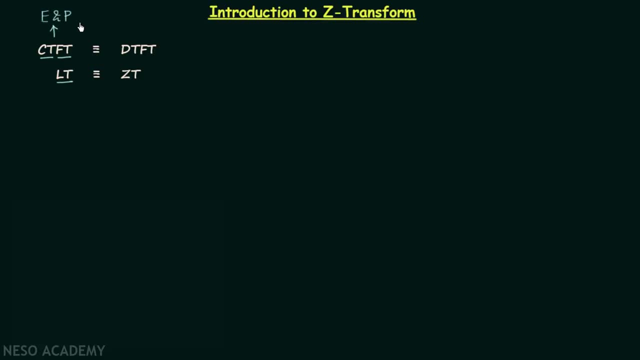 And power signals only, Whereas Laplace transform will exist for energy signals, power signals and also for neither energy nor power signals. But Laplace transform will exist for any NP signals, up to certain extent only Now, if you remember the previous chapter we had discussion on: 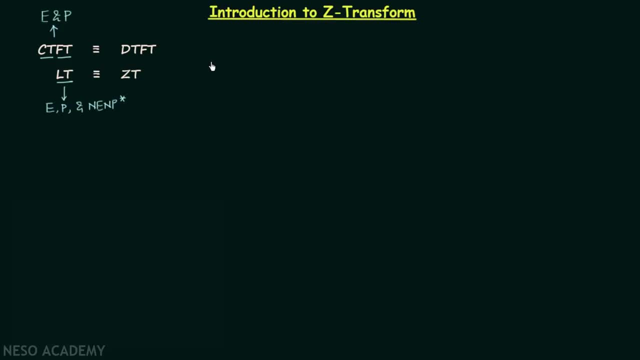 discrete time signals and systems and like CTFT we have DTFT that is in discrete time Fourier transform, and we use DTFT to convert discrete time domain signals to their corresponding frequency domain representations And we use it to analyze the discrete time signals. So DTFT is equivalent to CTFT and Z transform is equivalent to CTFT. 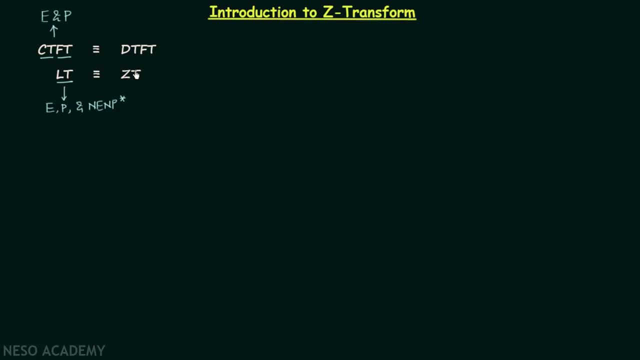 So DTFT is equivalent to CTFT and Z transform is equivalent to CTFT, Laplace transform and Z transform is the general case of DTFT and we use Z transform to analyze the discrete time systems. We can comment about the stability, causality etc. of a discrete time. 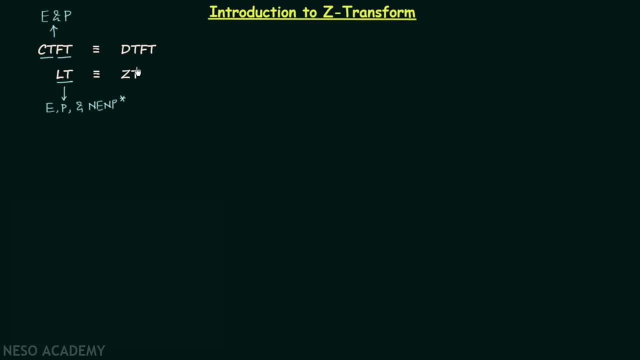 system using the Z transform. Now let's talk about the existence. Like CTFT, DTFT will exist for energy and power signals only, whereas like Laplace transform, Z transform will exist for energy signals, power signals and also for neither energy nor power signals, but it will exist for any NP. 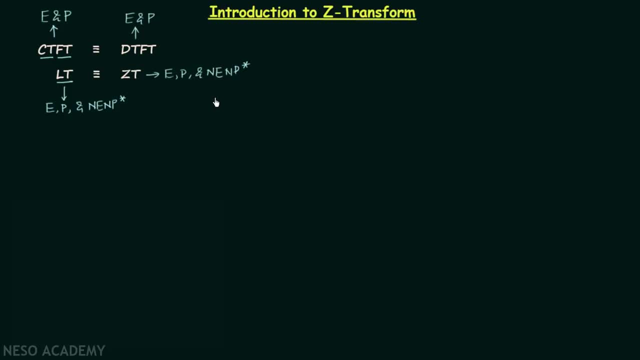 signals up to certain extent only Now out of DTFT and Z transform. we will first have discussion on Z transform And once we are done with Z transform we will move on to discrete time. Fourier transform: Now let's begin our discussion on Z transform And I will first give you the transform. Let's say there is. 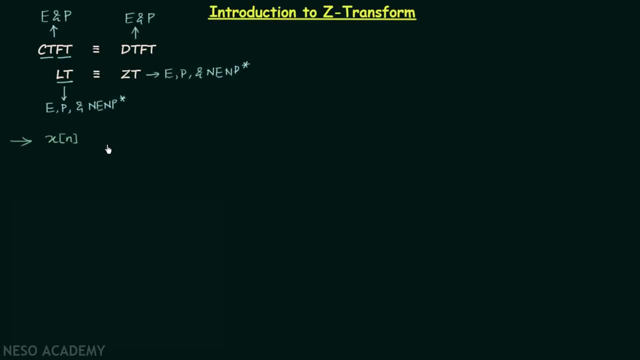 a discrete time signal, xn, and we want to calculate its corresponding Z transform. So we will perform the Z transform on this signal. and let's say its Z transform is uppercase X inside the bracket Z. So when we perform the Z transform of this signal, we have a new signal which is xz. Now when we perform the inverse, 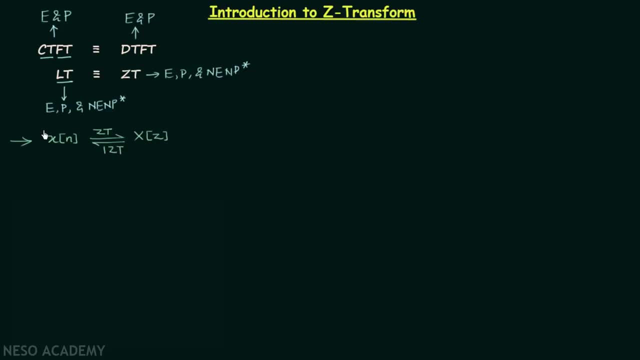 Z transform on this signal, we will have the original discrete time signal, xn, And therefore we call xn and xz as the Z transform pairs. Now to calculate xz, we will perform the summation from n, equal to minus infinity to plus infinity, the discrete time signal whose. 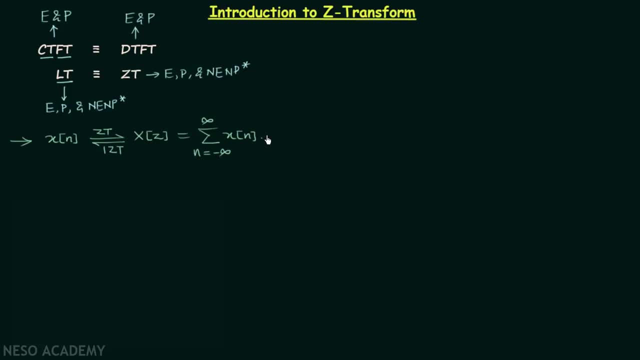 Z transform we are calculating multiplied to z power minus n. Now the summation part is clear. We are performing the summation from n equal to minus, infinity to infinity, And in this part we have the discrete time signal whose Z transform we are calculating. And then we 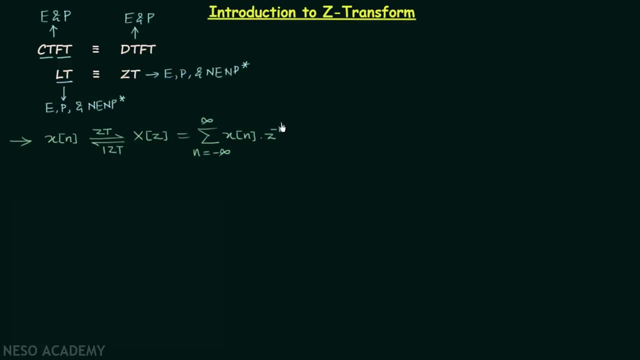 have Z power minus n. This n is an integer. It is an integer And Z is a complex variable. It is a complex variable And z is equal to r multiplied to e power, j, omega. This is the polar form of the complex variable z. Now this r is the magnitude of the complex variable z, So r is equal to mod z. 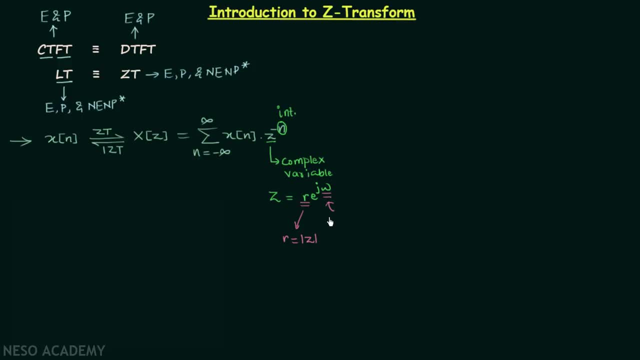 And this omega is the complex argument From this polar form, we will have a polar plot like this. You can see that we have a circle because when we change omega slowly, slowly, r will remain same and therefore we have a circle like this. Now we will talk about bi-directional Z. 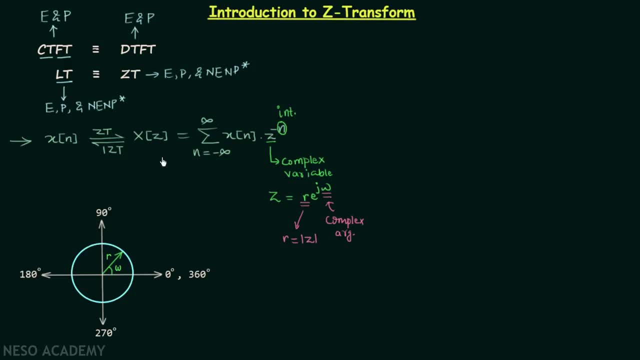 So we have the z transform and the uni-directional Z transform. This z transform I have written is known as bi-directional z transform. We are calling it bi-directional z transform because you can see that we are performing the summation from n equal to minus infinity to plus infinity. 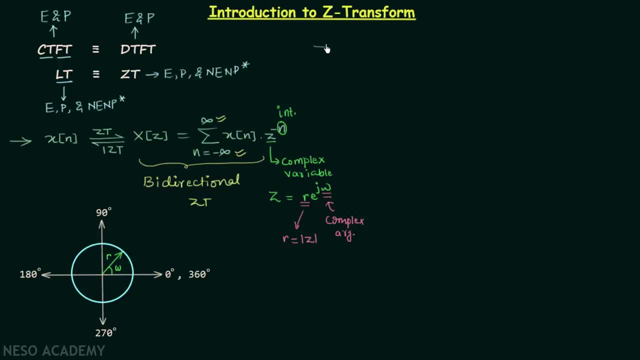 Now, if we perform the summation from n equal to zero to plus infinity, then we call the z transform uni-directional z transform. So this one here is known as uni-directional z transform. Now, to implement what we have discussed till now, let us solve one example. 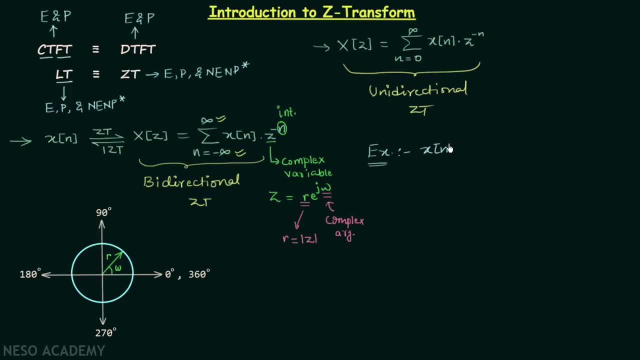 In this example, the discrete time signal xn is equal to a power, n multiplied to un, and we are required to calculate the corresponding z transform along with the region of the z transform. So let's move on to the solution of this example problem. Discrete time signal xn is equal to a power. 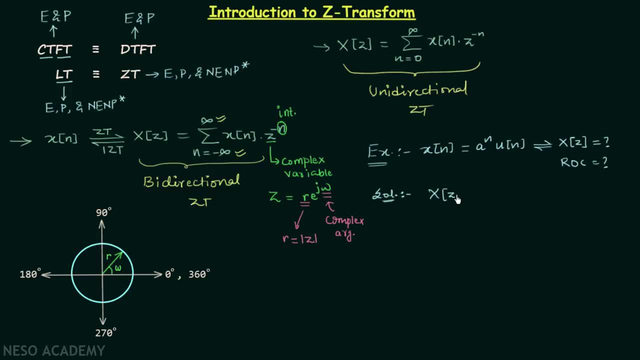 n, un. therefore the corresponding z transform according to this is equal to summation, n equal to minus, infinity to plus infinity, xn and xn is equal to this. So we have a power n multiplied to u And because of u, we will perform the summation from n equal to zero to infinity, because for all, 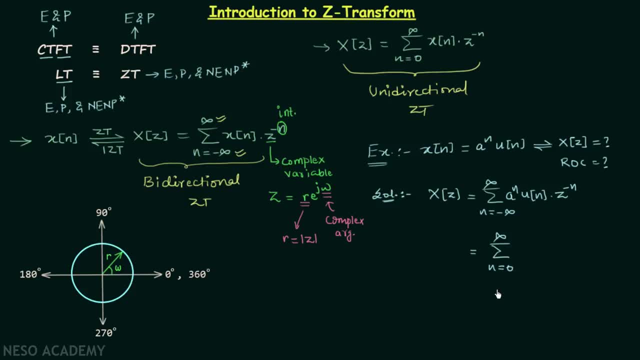 the values of n which are less than zero. we are going to get zero because of un, So we will focus on summation from n equal to zero to infinity. And we have summation of a power n multiplied to z power minus n. Let us write a power n multiplied to z power minus n as a multiplied to z power. 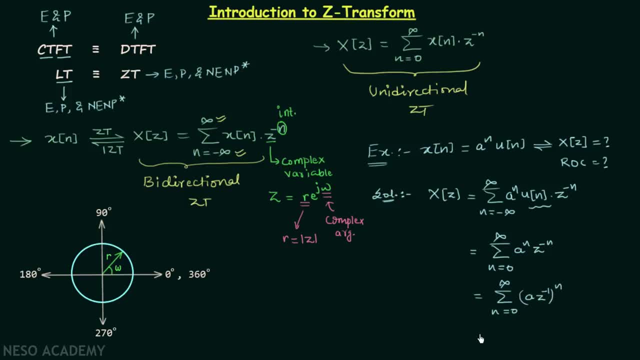 minus 1 power n. Now, when n is equal to zero, we will have one, because a multiplied to z power minus 1 power zero is equal to 1.. So this is our first term and to get the second term we will put n equal to 1.. So we have a multiplied to z power minus 1.. Similarly, the third term. 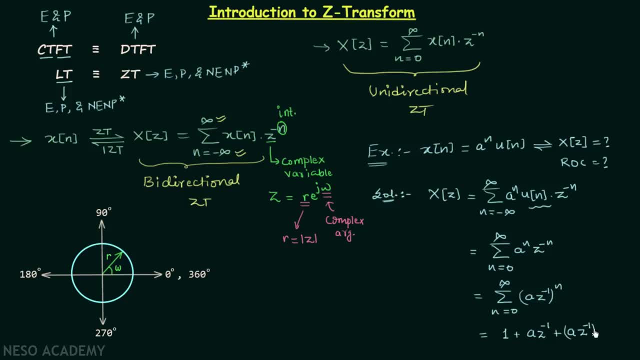 will be a multiplied to z power minus 1, square, all the way to the term which is obtained when n is equal to infinity. Here you can see that we are having the sum of infinite gp, The common ratio we are getting. common ratio we are getting is equal to a multiplied to z power minus 1, and we know the. 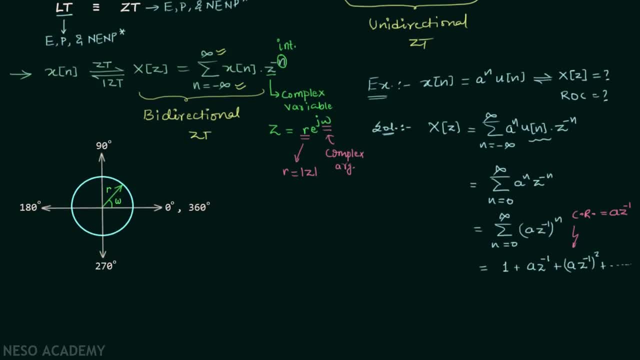 sum of infinite gp is equal to the first term divided by 1 minus common ratio. So sum of infinite gp is equal to infinite gp is equal to the first term divided by 1 minus common ratio, And we can use this formula when the mod of common ratio is less than one. So let's use it to solve our summation. 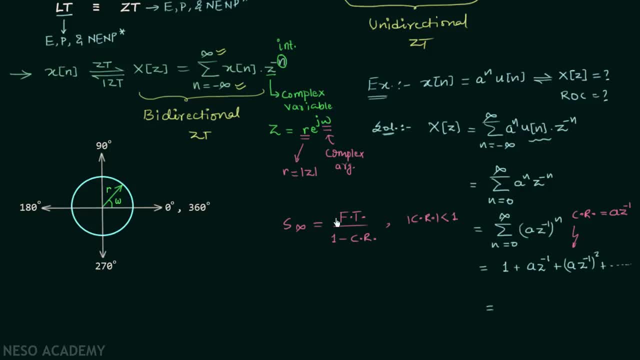 We are having one as the first term, So we will write one in the numerator divided by one minus common ratio, And we are saying that the common ratio is a multiplied to z power minus 1.. So this is what we have as the z transform. But we should also be vigilant about this condition here, That is, mod of the common. 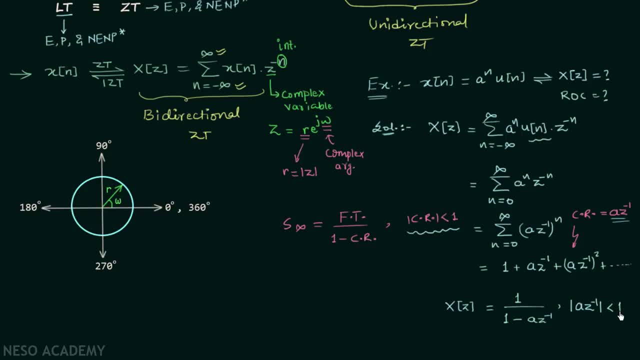 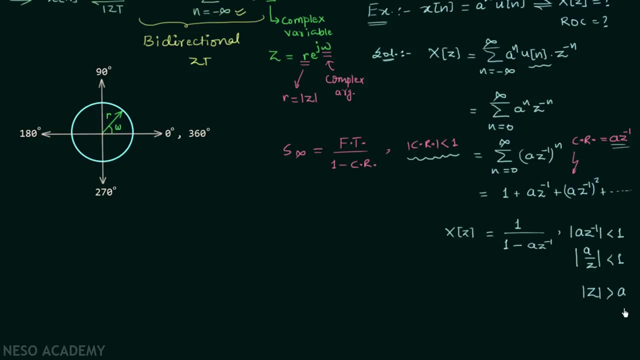 ratio, a multiplied to z, power minus 1, should be less than one. From here we can say that mod a over z is less than one, And from here we can say that mod z is greater than a. And this is our region of convergence. mod z is equal to r, the magnitude of the complex variable. So ROC is equal to. 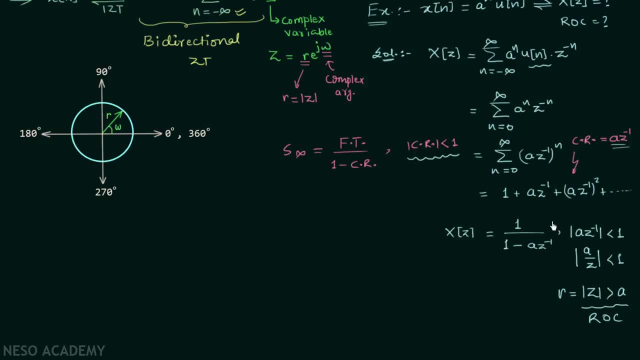 r greater than a And hence the Z transform we have calculated will exist only when r is greater than a. Now we will quickly plot the ROC. This is our z plane, And we will first draw a circle having the radius equal to a, According to the condition we are having. 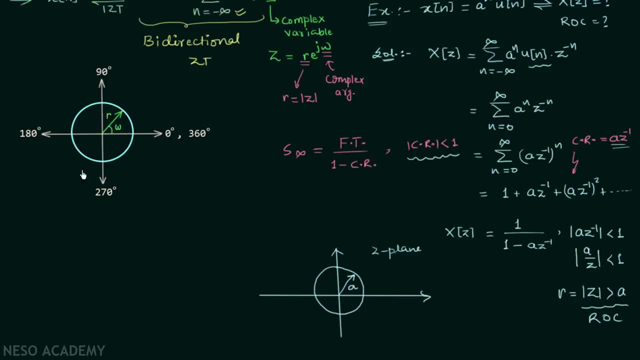 here r should be greater than a. This means the region of convergence is all the region out of the Z plane, Outside this circle- And we know the significance of region of convergence- The Z transform will exist only within the region of convergence, Outside region of.